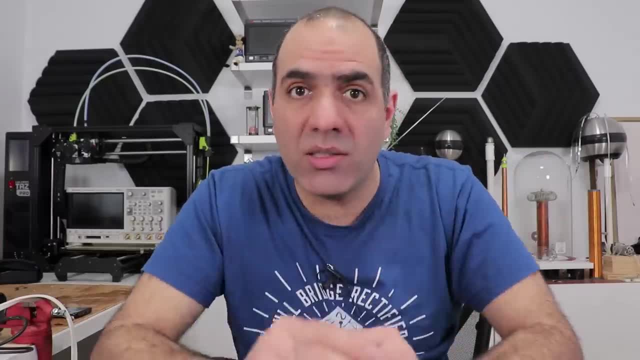 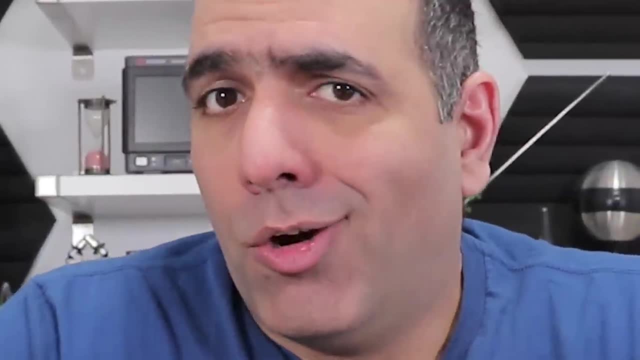 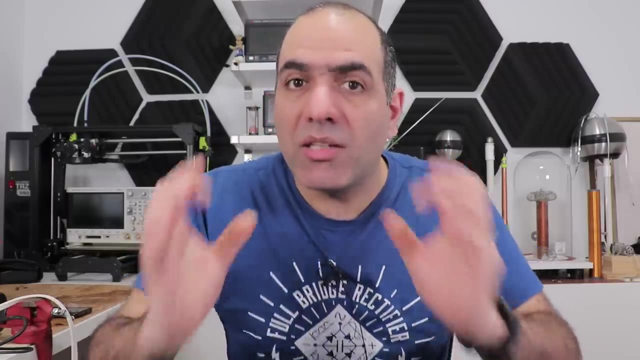 Here. I just want to surf the surface and talk about what it does, so we can design circuits with it. Semiconductor diodes are amazing. though You think they just rectify, Well, think again. There are millions of different types- maybe around 10, but they are all made based on. 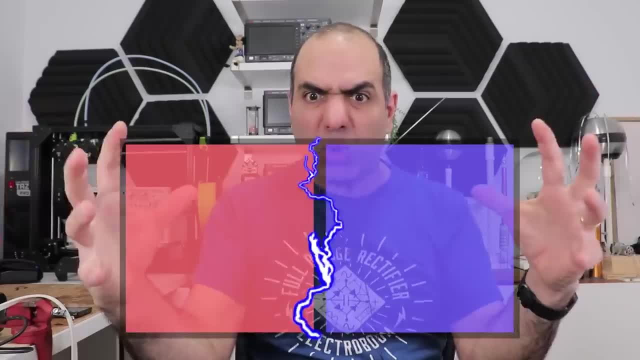 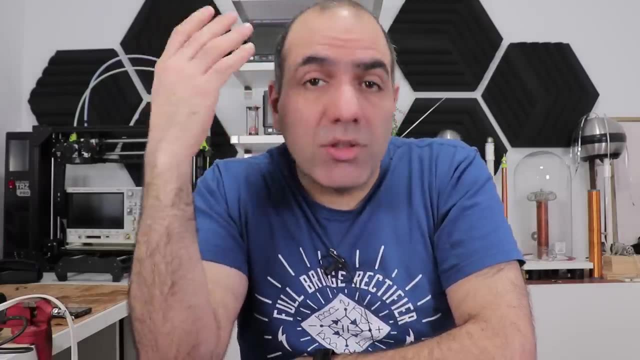 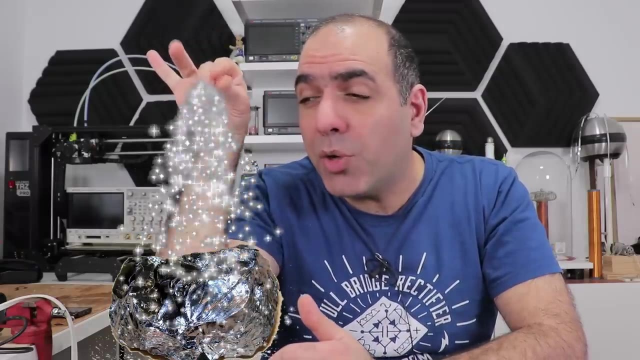 the same concept: Two different materials are fused to each other and the junction between them has magical properties. Fine, I go a bit deeper. Semiconductors are materials typically made of silicon crystal. that we dope them with small amounts of impurity, And if you 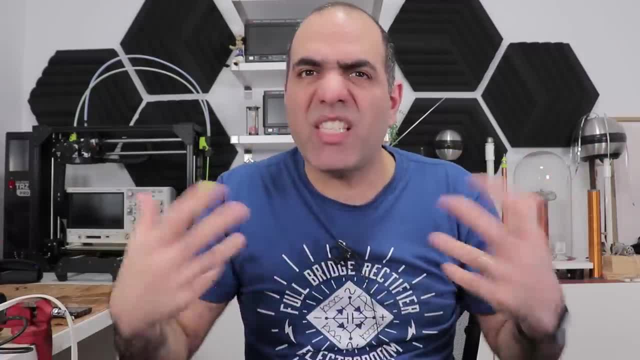 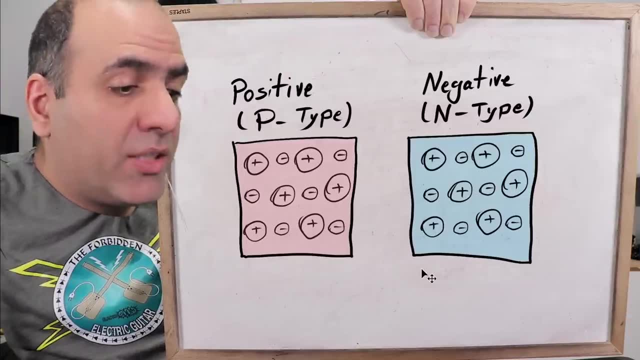 use some of these, depending on the type of impurity. we get positive or negative semiconductors. As their name suggests, they are conductive. they are electrically neutral, of course, but if we fuse the two types together, the p-type will happily pull electrons from the 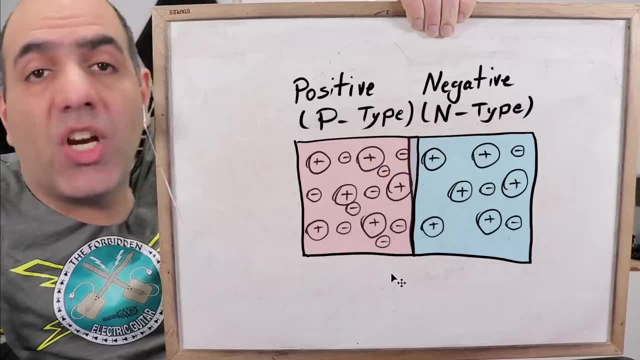 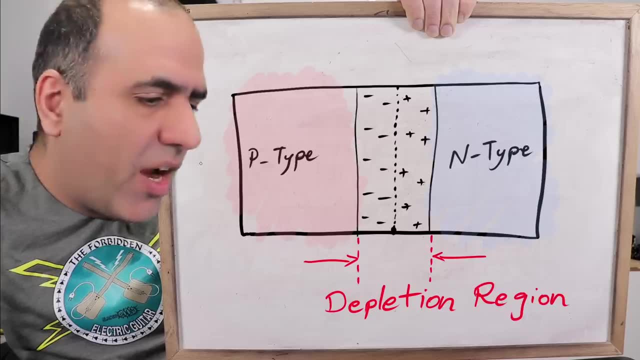 n-type which is happy to give them right at the junction. This creates a small region of charge imbalance called depletion region. So this means if we decide to put a positive voltage on the p-side, we have to separate it right on the junction. And that's what. 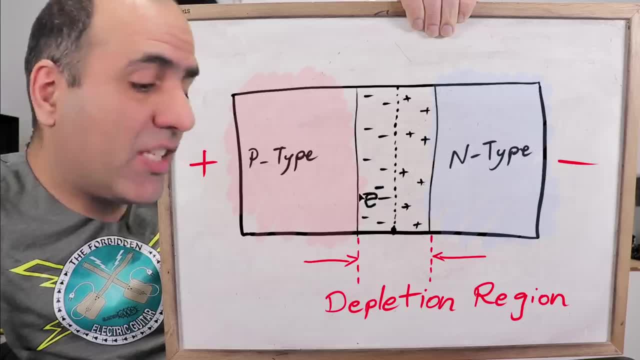 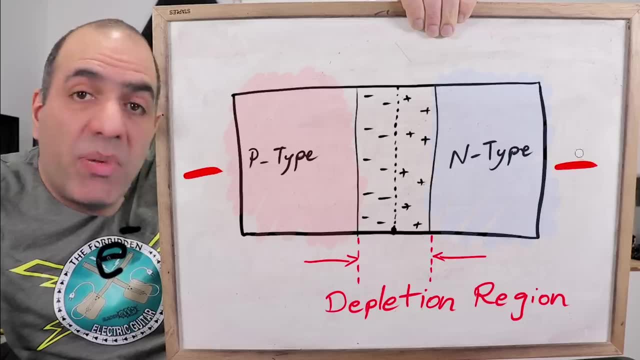 happens, The electrons and electrons collide and they become like a group. and if we separate and suck electrons out, p gladly takes electrons from n and the negative terminal and current flows with low effort. But if we flip the voltage across the p-n junction and try to force electrons into p, it won't want to pass. 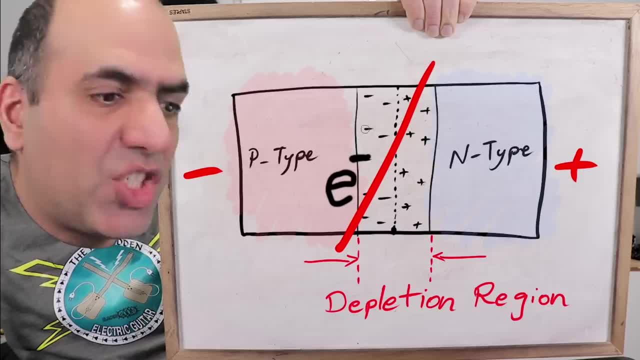 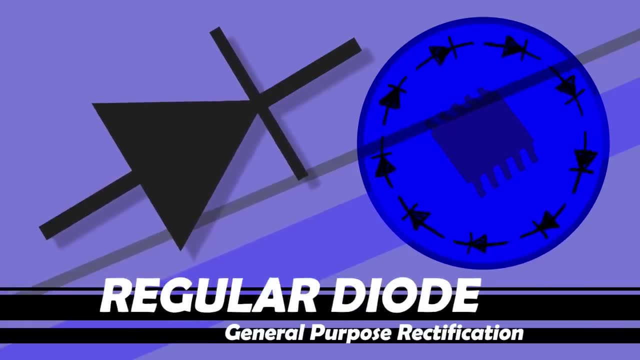 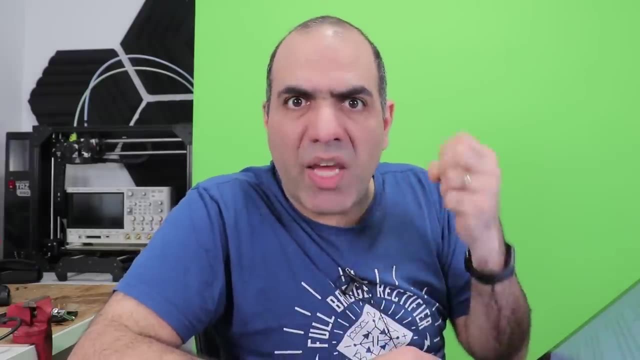 electrons into n. That's not their deal. The p-n junction blocks the electric current, so we have a diode. Just try to remember the p and n behavior, because it will later help you understand the behavior of all semiconductor components. p wants to suck. 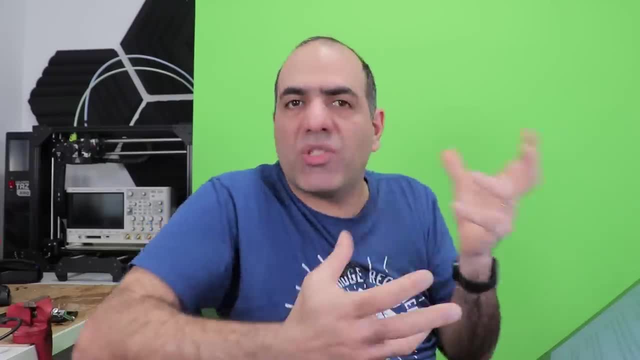 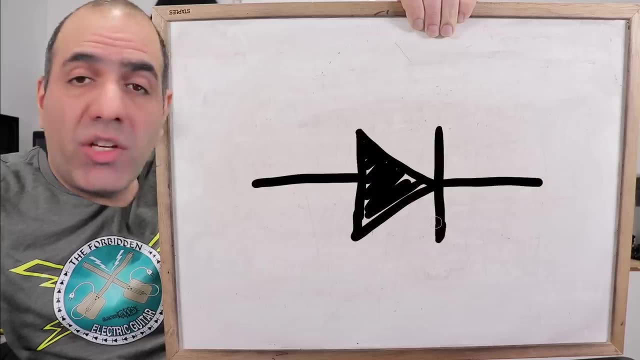 electrons from n and n only. It doesn't want to suck electrons from the power supply. This is a marriage contract. only p and n got into. Diode is generally shown with this symbol like an arrow indicating the direction the current can flow. 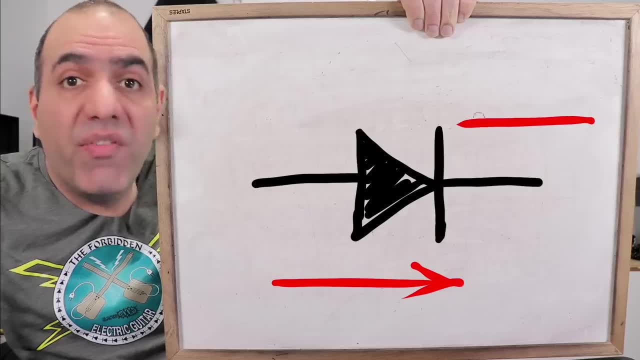 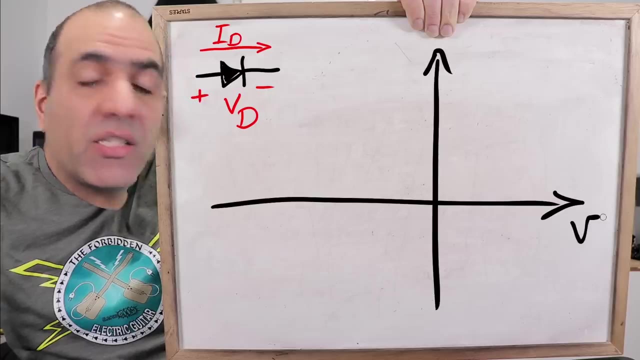 Which is the reverse of flow of electrons, and how a reverse current will be blocked by this wall. This is also the symbol of a general-purpose diode. You'll see that different type of diodes will have different symbols. Now let me show you the ideal behavior of a diode. x-axis is the voltage across the diode and y is 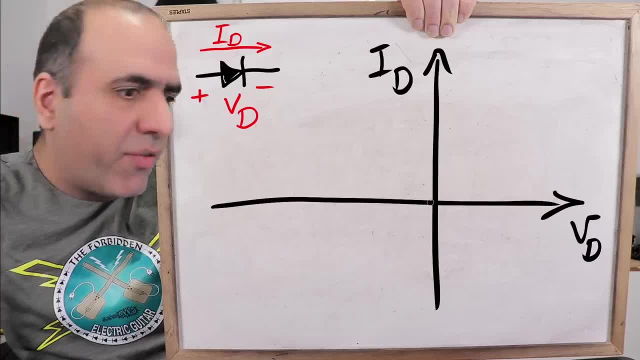 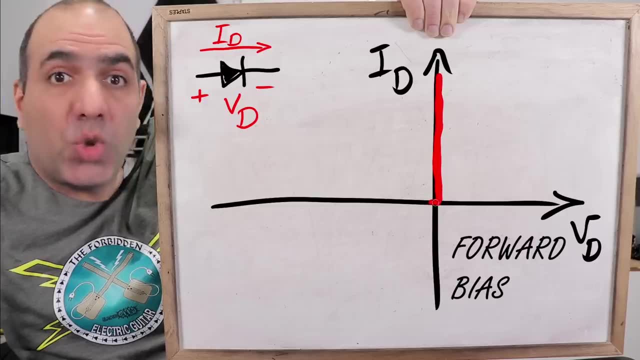 the current through it. If the voltage across it tries to get positive or the diode is forward biased, it turns on like a switch and lets through any amount of current, Like this, Like a short circuit. But if the voltage is negative or the diode is reversed, 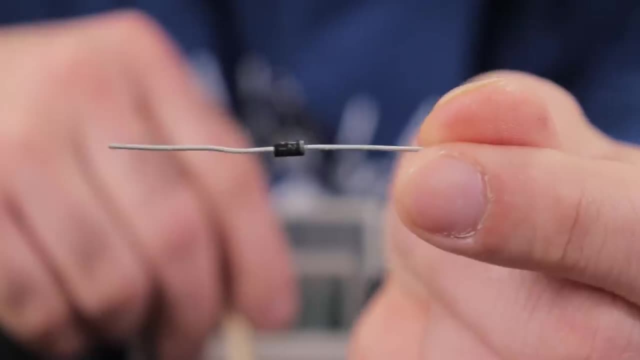 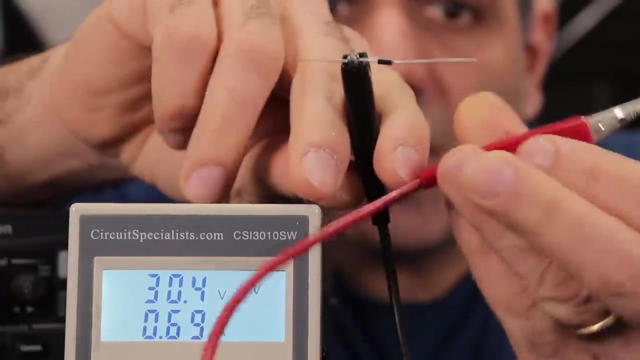 biased, it blocks and there is zero current. Here's a typical through-hole diode. You see, the gray line here indicates the direction of the diode. You see, if I try to put the diode in reverse, the current reading is a bit off It. 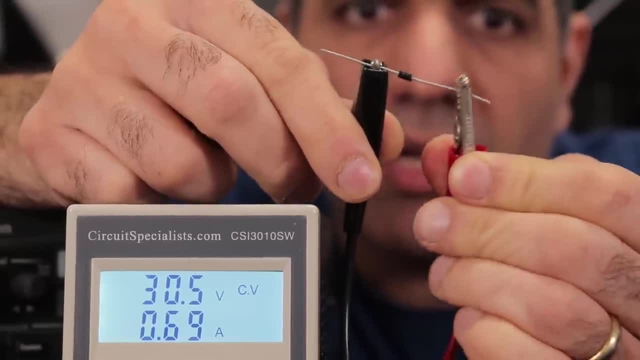 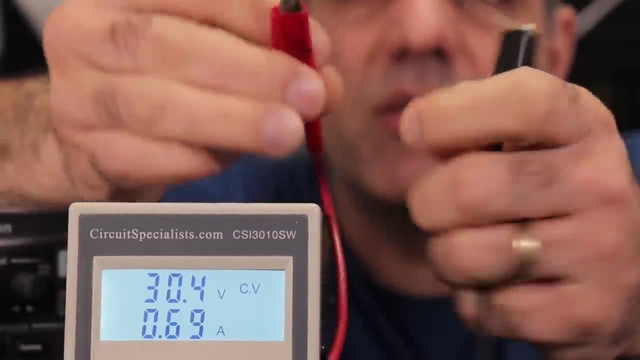 doesn't conduct and there is no extra current from the power supply. But if I flip the voltage, see it is starting to conduct like a short circuit. Oh Burned. We must not exceed the power rating of the diode, So I'll place a 10k resistor. 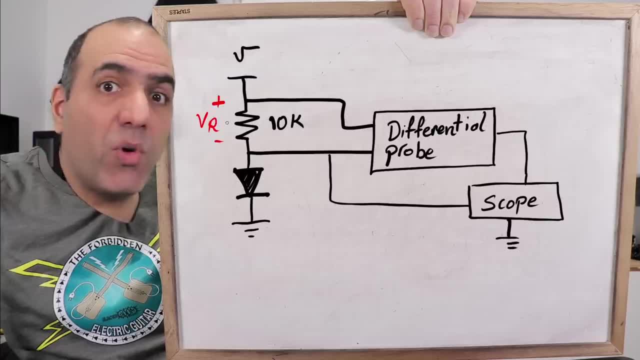 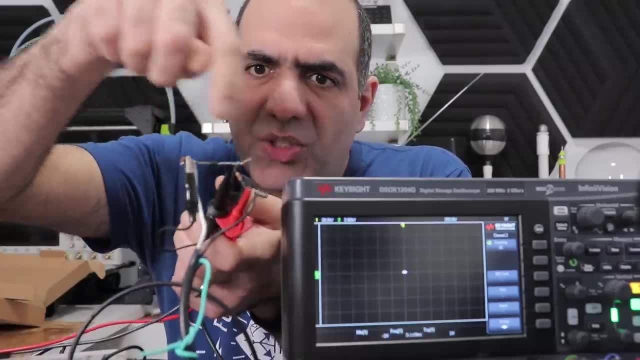 series to it to limit the current. and now we can measure the voltage and current through the diode For current. I'll just measure the voltage across the resistor. I don't know if you can see my resistor and diode in this mess of. 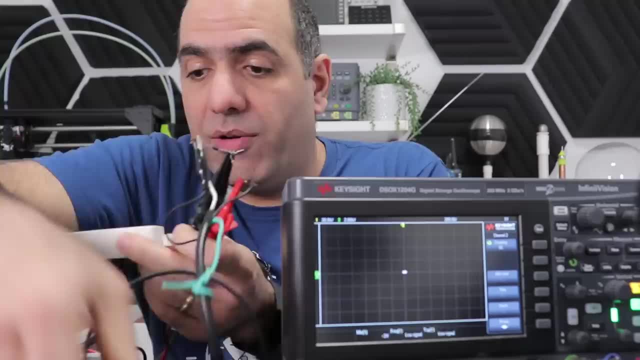 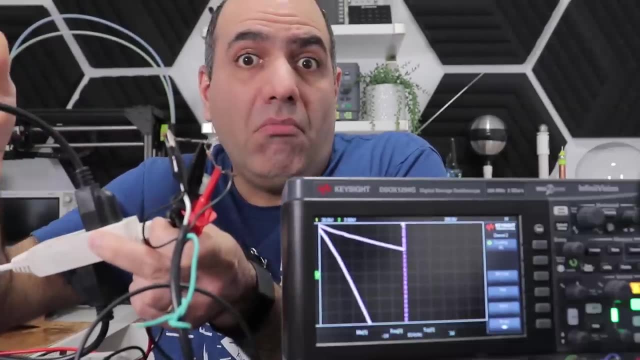 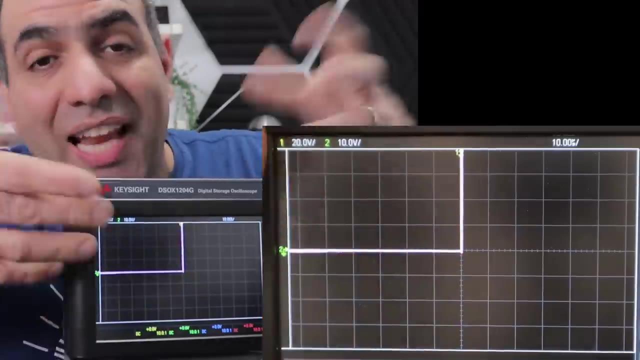 probes And for my AC power supply. of course, I use the power line. Hmm, It's fine. I put my scope in XY mode, X being the voltage across the diode and Y- current through it, and it acts like a diode for negative voltages. there is no current and for 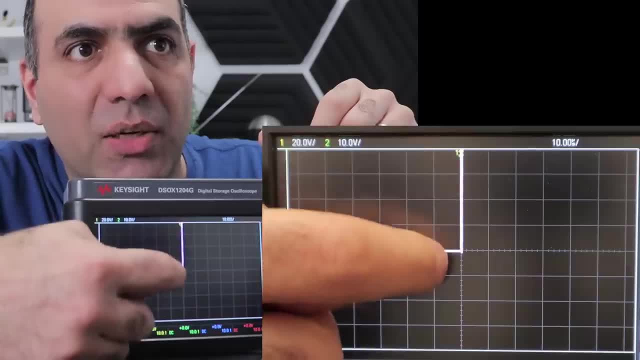 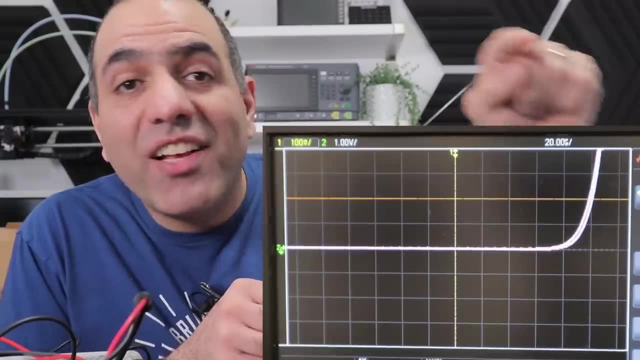 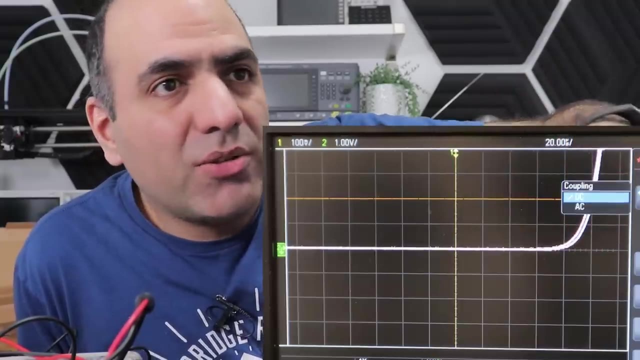 positive voltages. it acts like a short circuit. there is current but no voltage, or is it? let's zoom in on voltage. see, this is a real, non-ideal diode. it takes a little bit of voltage before the diode starts conducting, which is different from diode to diode, and we can assume it to be around 0.6 volts for decent. 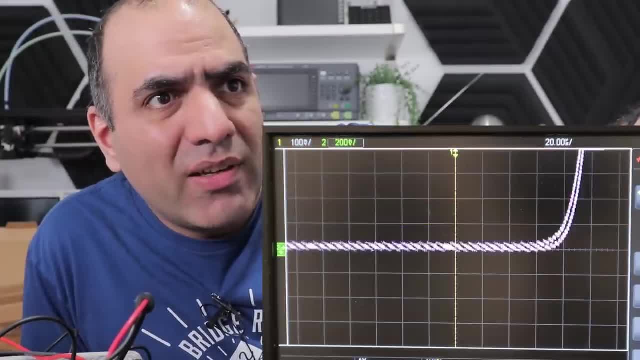 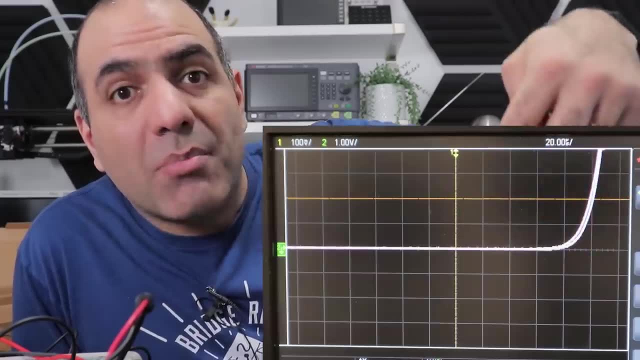 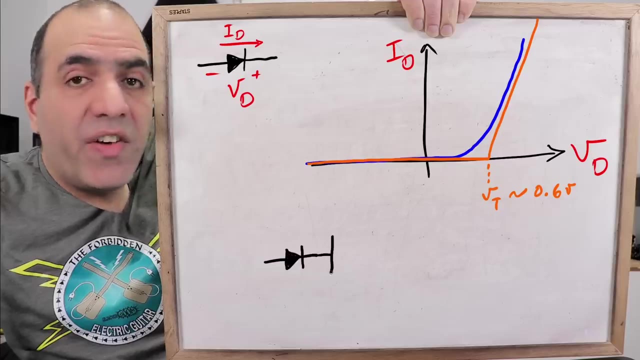 amount of current, but it's actually a little less for a smaller current and a little bit more for higher currents and after that initial voltage the current ramps up. so we can approximate a diode's behavior like this: an ideal diode in series with a reverse 0.6 volt, ideal battery we have to overcome and a small. 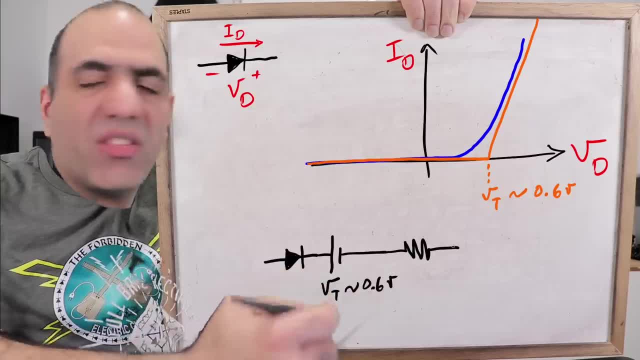 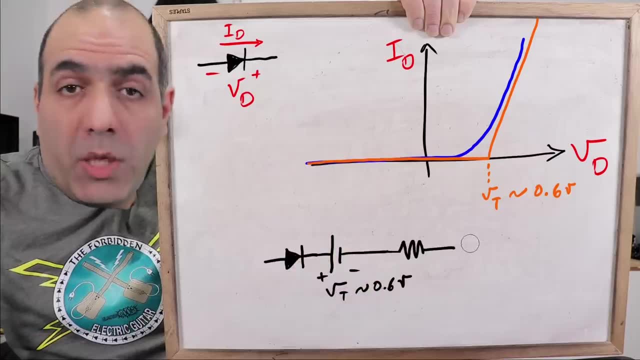 series resistance, or I do. when you use a diode, just understand that there is around 0.6 volts across it that can rise slightly when the current rises. we typically ignore this resistance for most applications because it's small, and we can also ignore this voltage if it is too small compared to the voltages in 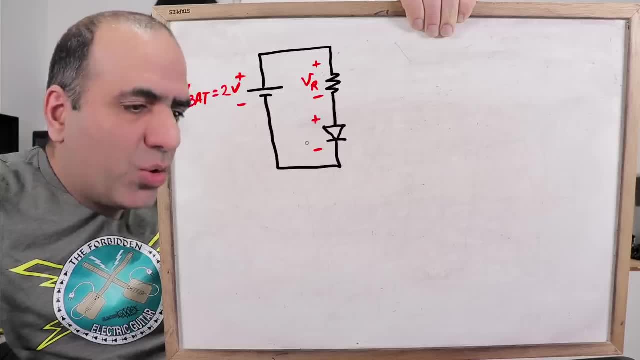 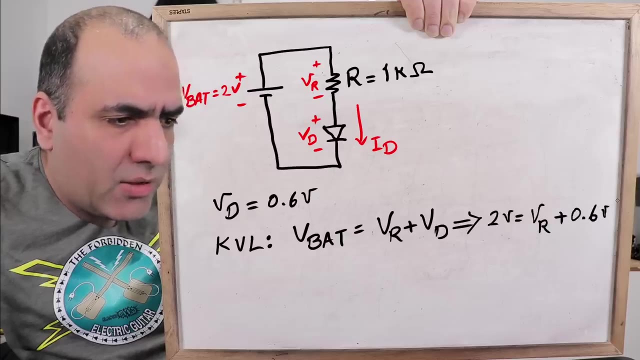 our application, like if they give you the circuit and ask you to calculate the current. you can just assume the diode voltage is 0.6 volts, write a KVL as V bat equals resistor voltage plus the diode voltage, or 2 volts is equal VR plus 0.6 and VR is equal RI, or 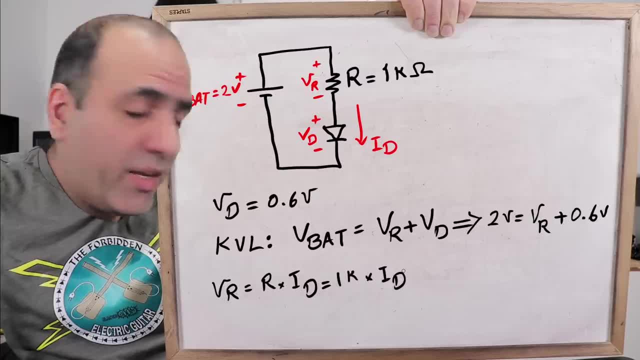 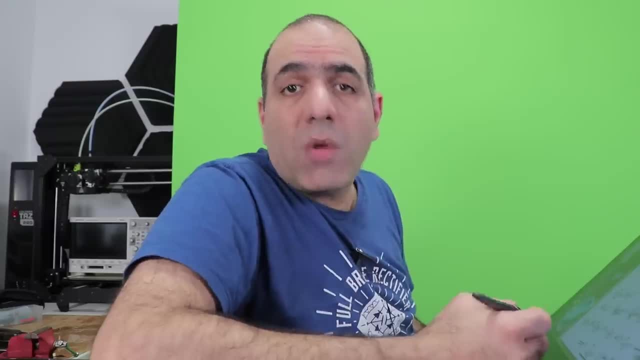 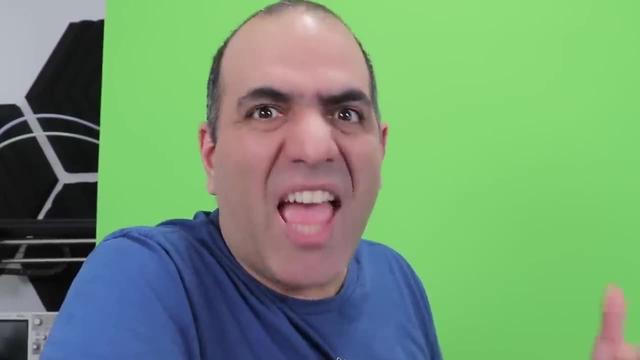 equal to 1 K times I. so I is equal to minus 0.6 divided by 1000, or almost 1.4 milliamps. and if they want it any more accurate, tell them to pull the soldering iron out of their butts, because nobody writes diode and accuracy in one. 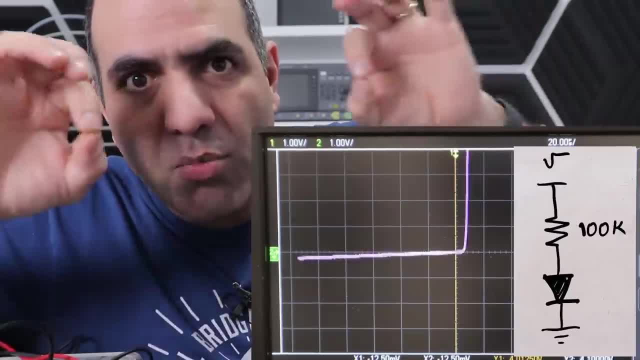 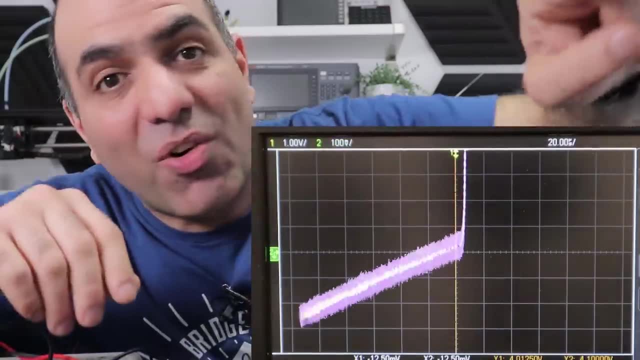 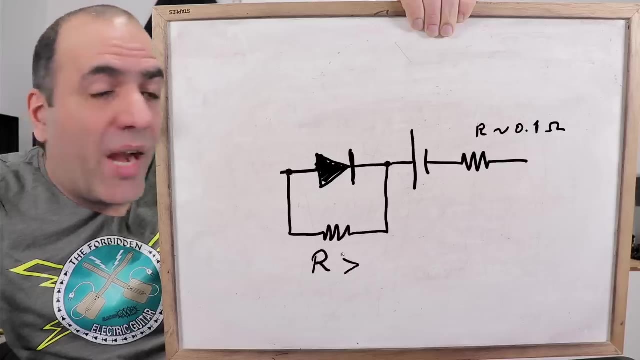 sentence. now we change the series resistance to 100 K for more precision and let's zoom in on the current. look at that. the current is not zero in reverse voltage. there is a very small leakage current in reverse so we can add a very large resistor across the diode to model it. 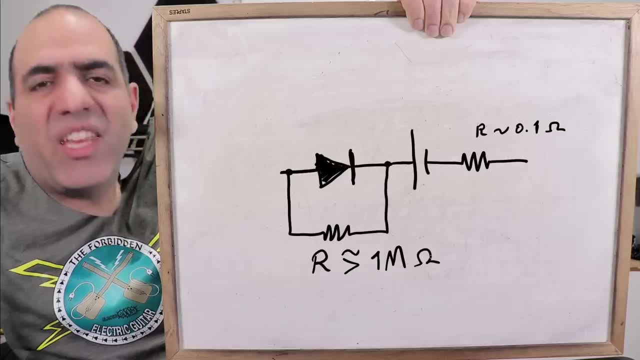 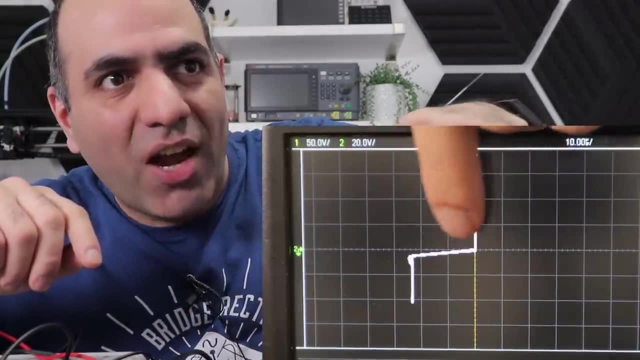 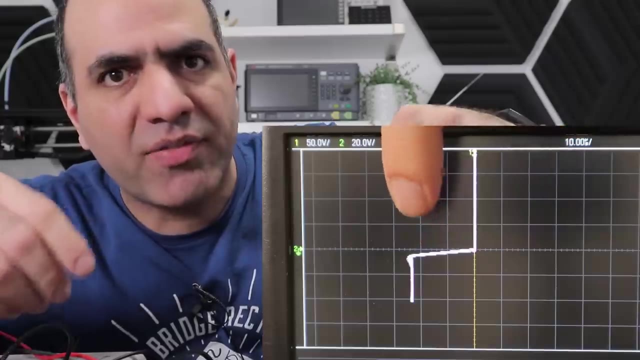 although the leakage current is typically so small, we can ignore it. this time let's zoom out on the voltage. look at that: the diode that's supposed to block current in reverse voltage is conducting large amounts of current when the voltage passes above some threshold, around 100 volts in this case, the voltage where current starts flowing is 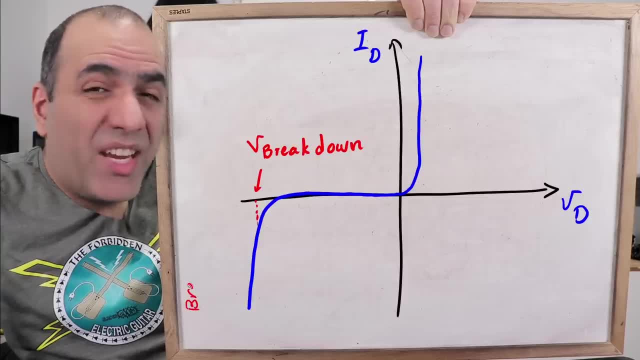 called the breakdown voltage and the region behind it is the breakdown or Avalanche region. if you push the diode too hard in reverse, it starts conducting. that could be destructive to the diode. the reason diode dies here is because you would have very large reverse voltage and current through it, which 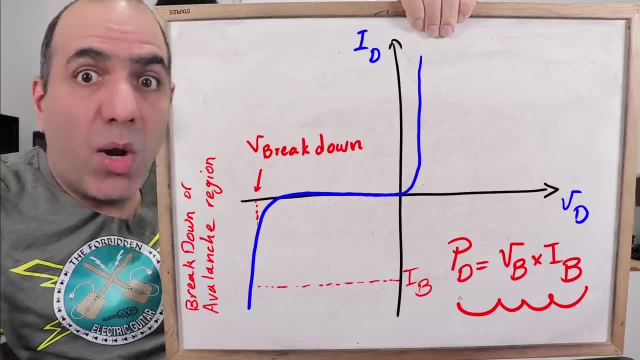 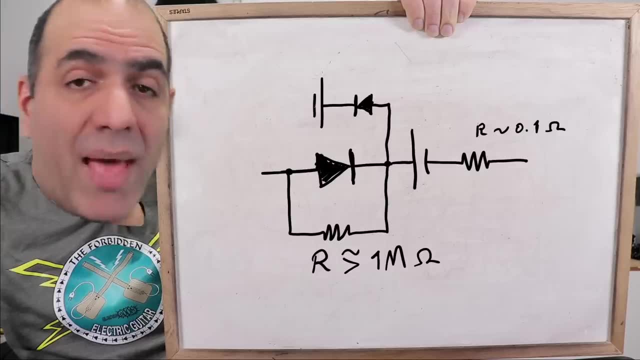 results in very large power, drop it up quickly and blows up unless you get out of that region very quickly. That can be modeled with a reverse ideal diode and a battery with breakdown voltage value. You have to be larger in reverse than this voltage for the diode to 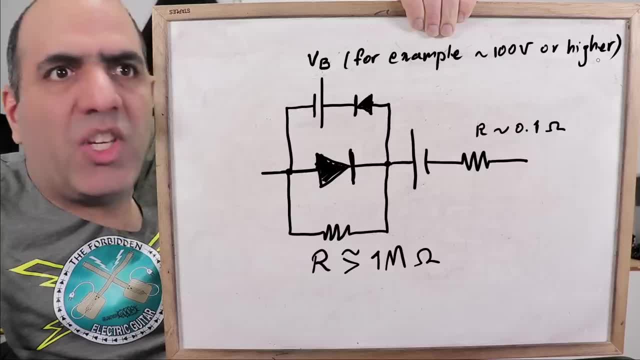 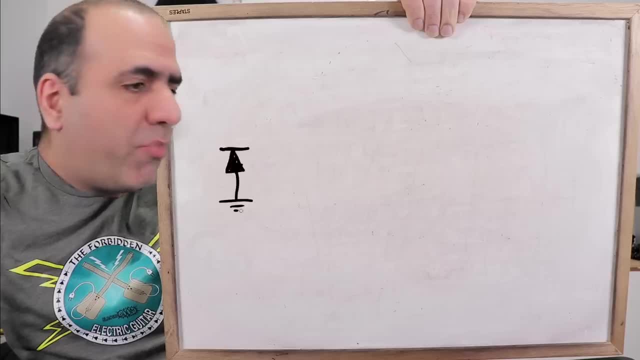 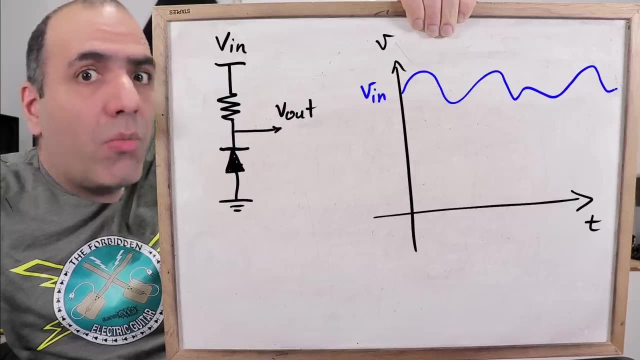 conduct backwards. We typically ignore this because we keep below that voltage level because that's not a desirable effect. Until it is, We can make use of breakdown voltage. If it is a reliable known voltage, we can use limited current through it and create an almost fixed voltage typically used as a reference. 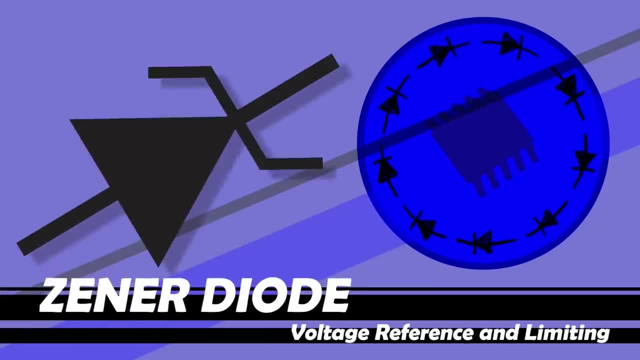 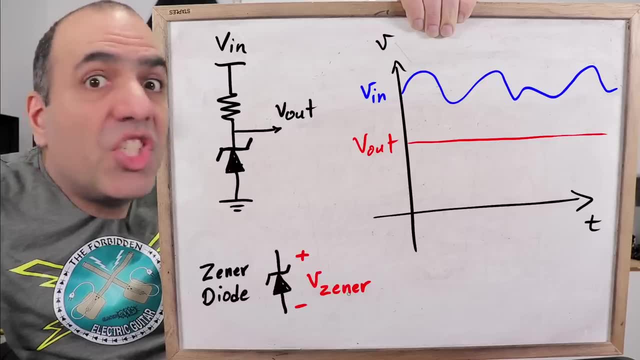 voltage, And so we make something called a Zener diode. Zener diodes are designed to have specific breakdown or Zener voltages like 1 volt, 5 volt, 10 volt or whatever. In a circuit like this, a Zener diode. 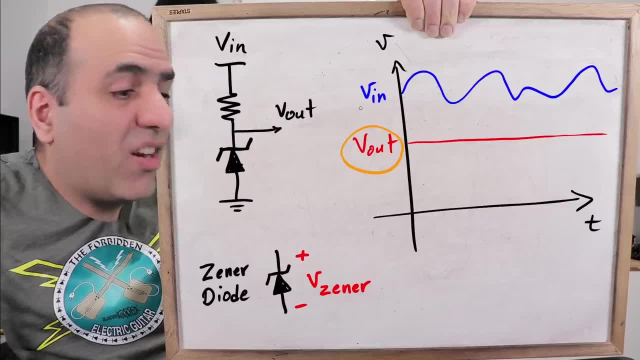 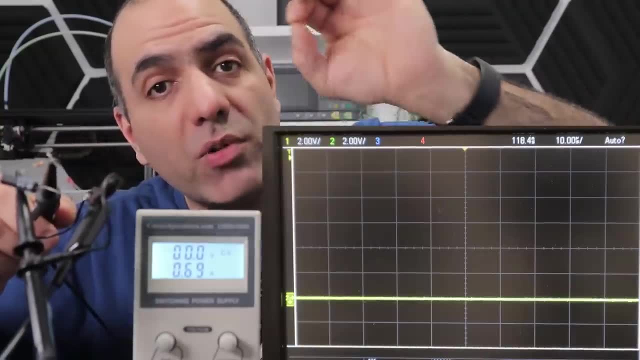 will clamp the voltage close to its breakdown voltage, regardless of the input voltage. Well, as long as the input is higher than the Zener voltage. Here I have a 5 volt Zener diode series with some resistance, and if I raise the 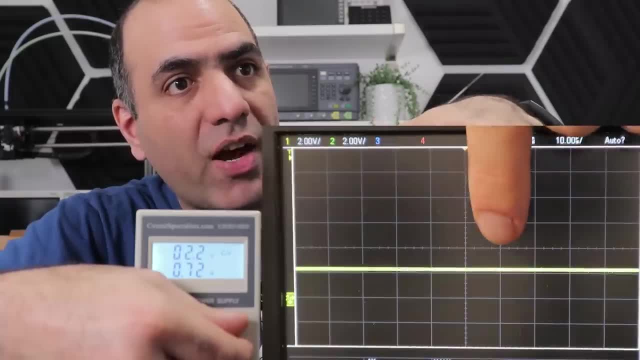 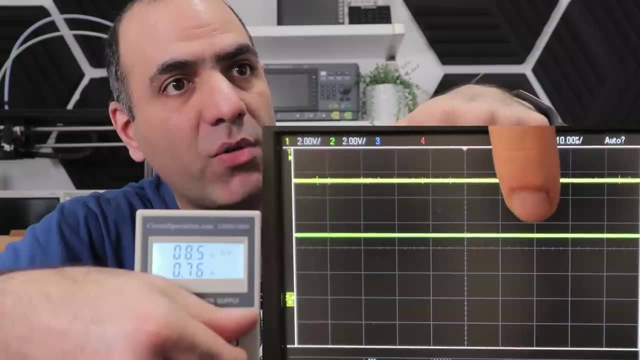 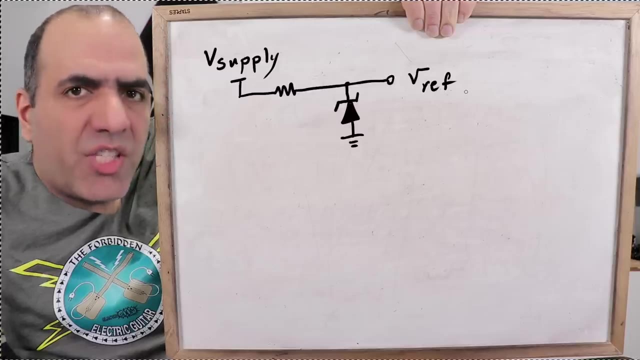 supply voltage. you see the Zener and supply rise together until around 5 volts. Zener starts conducting. the supply rises, but the Zener voltage is clamped around 5 volts. Zener's can be used to generate fixed voltages as. 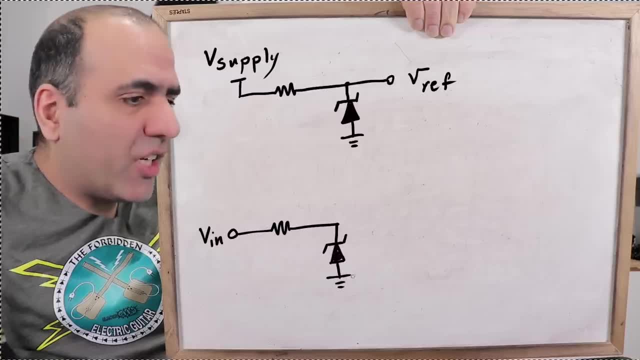 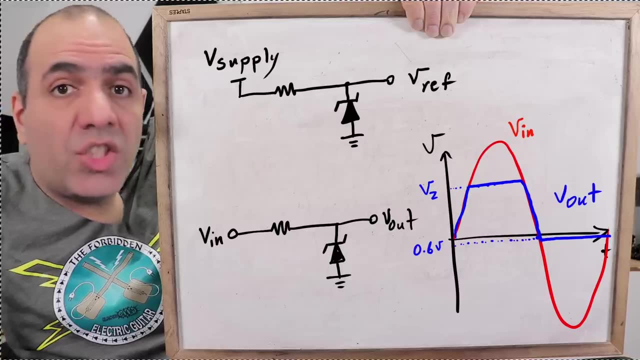 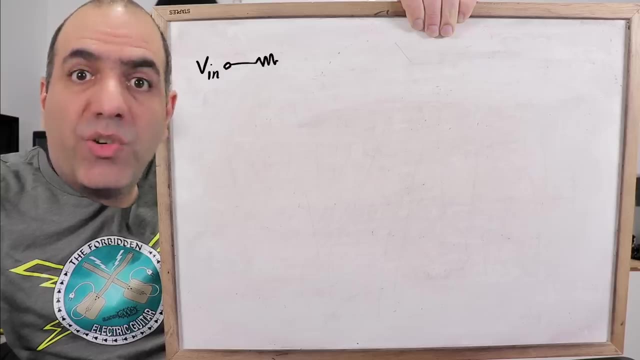 references, or they can be used to protect the circuit against high voltages By clipping the large voltages like this. In case of protection, they typically call such diode TVS or transient voltage suppressors, which are much faster to react to transients and are more powerful. A single one called a 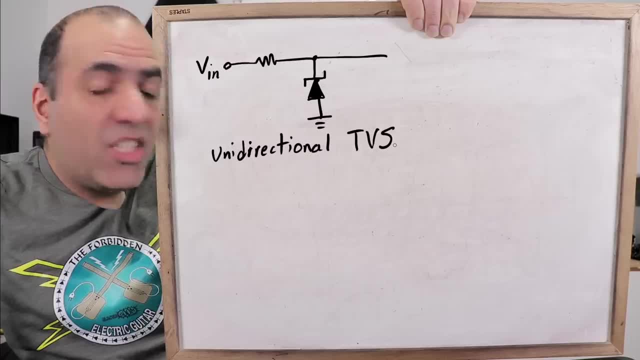 unidirectional TVS like this is placed in reverse on signal lines to clamp over voltage. like this, Two TVS diodes can be combined like this as one component called bidirectional. The first one is a single-signal TVS that can block the transient high voltage. 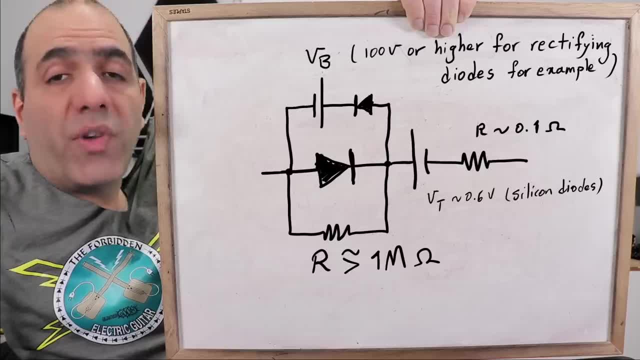 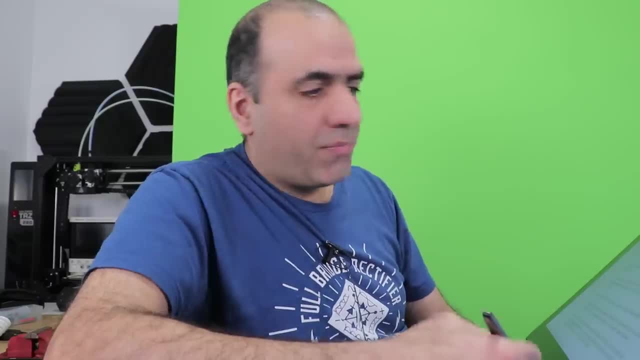 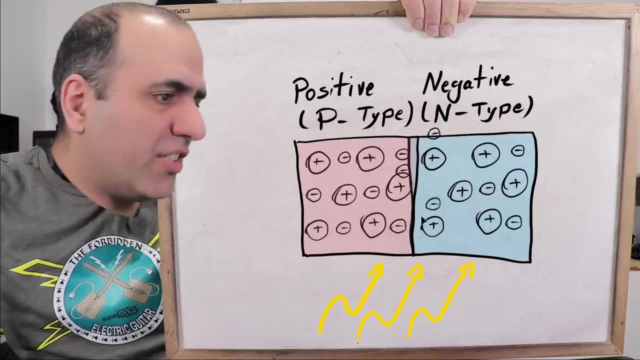 between a positive and negative breakdown voltage. But for regular diodes we typically ignore all these and usually keep it at this level, Except well, there is more. The thing is, if you shine a light on the PN junction, particles wiggle harder, sending more electrons from N to P, raising the voltage and 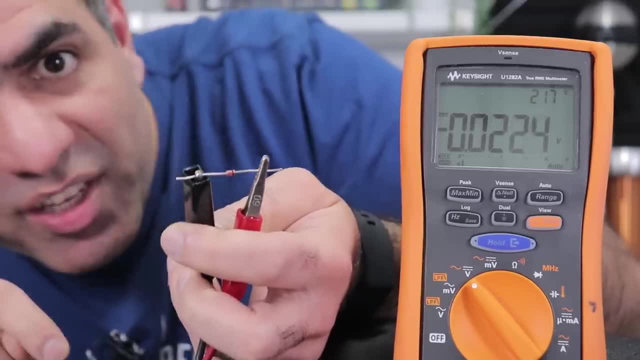 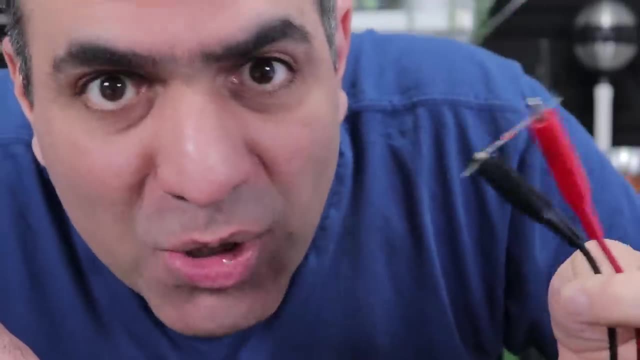 affecting the diode's behavior. Like this, diode's body is glass and the voltage is increasing, So if I shine a light on the PN junction, the voltage across it rises when I shine a light on it. But we made use of that too, So diodes can be light sensors or, as we call them, photosensors. 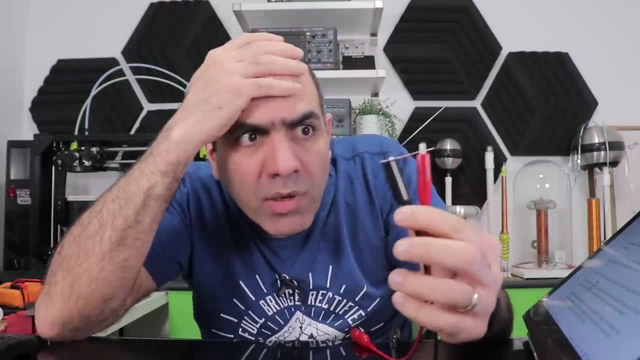 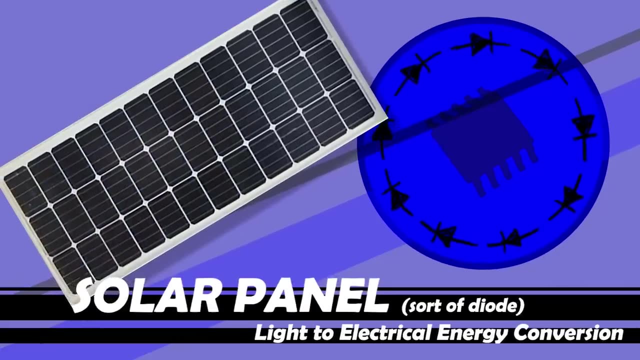 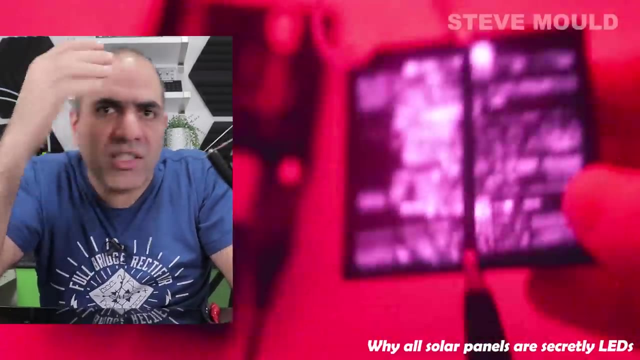 Did I mention? they make voltage when we shine light on them. If we play with the chemistry and make them more efficient, we can draw energy from them. And we have solar panels, Renewable energy- here we come. But, like Steve Mould mentioned in his video, if, instead of 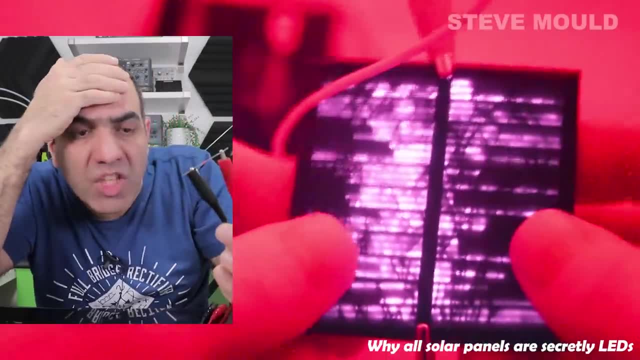 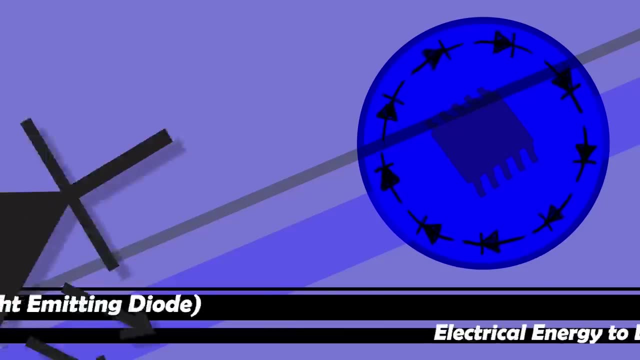 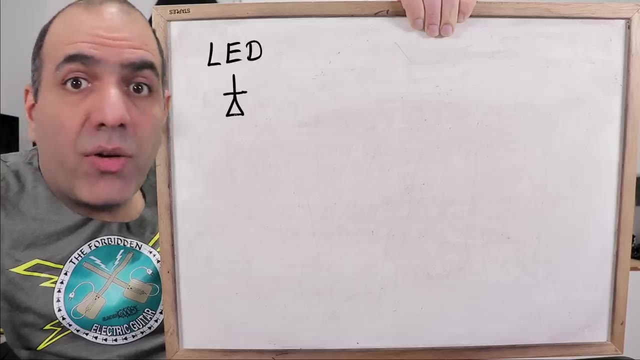 pulling energy from them. we apply a voltage across them. they create light in infrared. Now we mess with the chemistry again and make them produce visible light And we have LEDs- Efficient lighting. here we come. The only difference between LEDs and regular diodes is well beside the fact that they 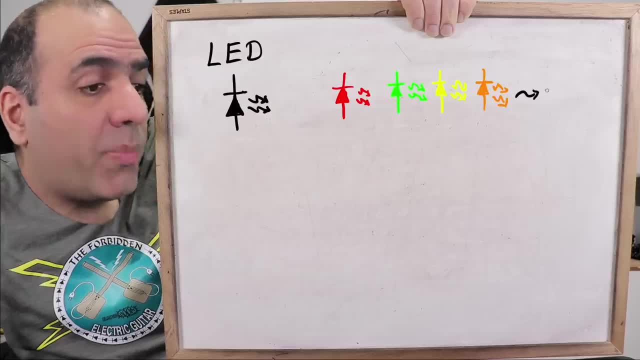 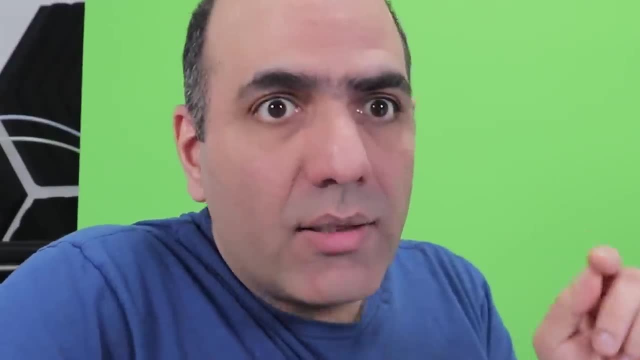 generate visible light, that their forward voltage drop is larger depending on their color. Otherwise they could also be used as a poor diode. Oh and remember when I said a diode blocks reverse current If you look at the PN junction. there the depletion layer acts like a thin layer of insulation, So the diode acts like a capacitor holding charge. The width of depletion layer depends on the reverse voltage, which means adjusting the reverse voltage. you can change the capacitance- A variable capacitance based on the voltage. 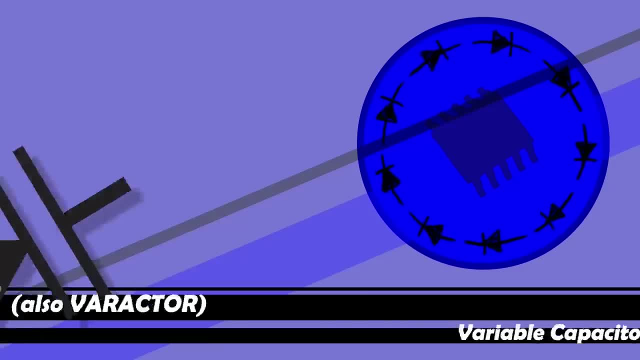 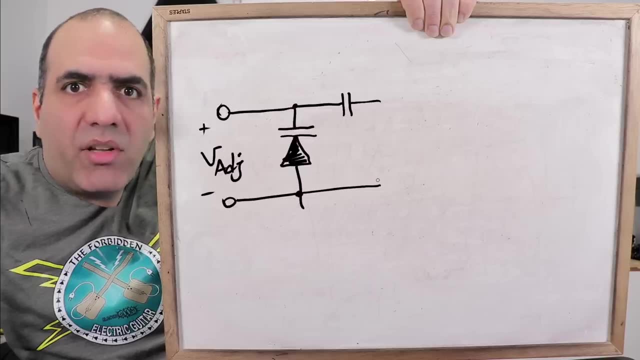 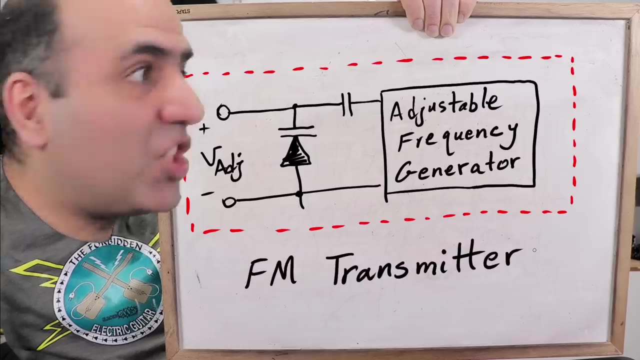 across it It's purpose. and you get a battery cap or a varactor Tuning the capacitance with voltage. you can create, for example, an adjustable frequency generator, Maybe to make an FM transmitter. Semiconductor diodes- man, they change the. 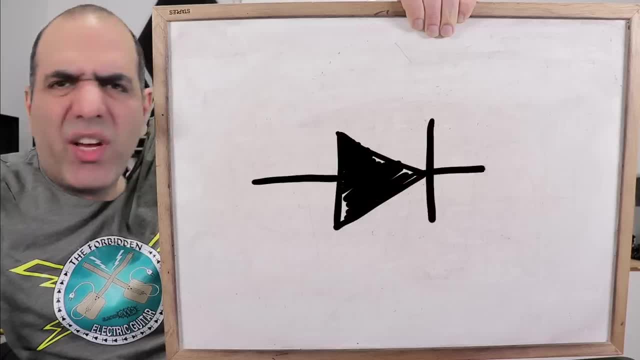 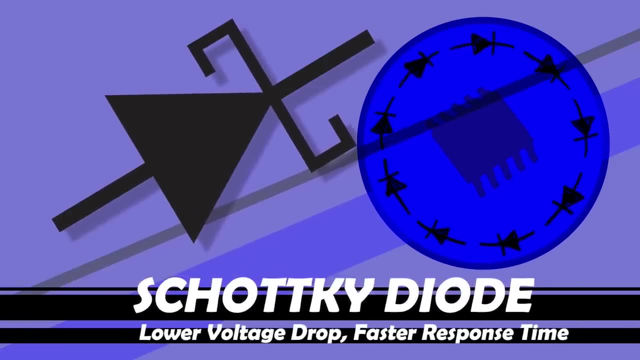 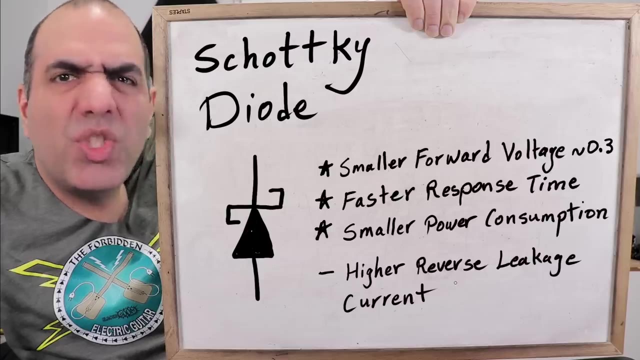 world. But mostly when we say diode we are referring to the regular current rectifying diode or its cousin Schottky diode, which has a much faster response time and lower forward voltage, so less power loss, But has a larger reverse leakage current, mostly used in switching power applications. 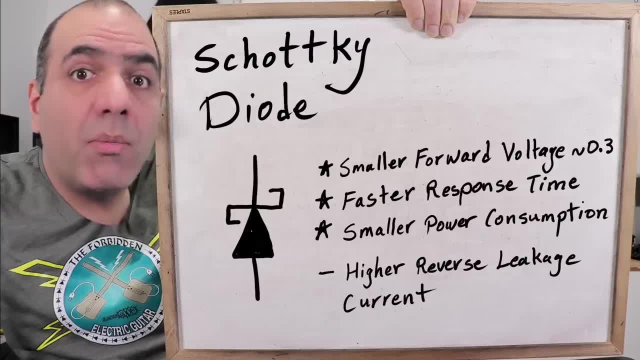 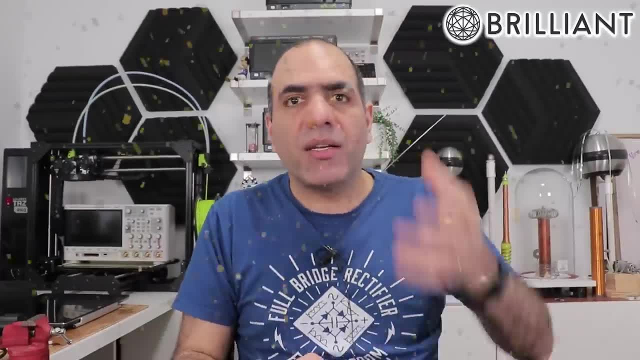 There are other types of diodes I care less about. What I care more about, though, is Brilliant the sponsor of this video. Brilliant man, just brilliant. It's an awesome tool for learning simple to complex STEM concepts of math, science and.